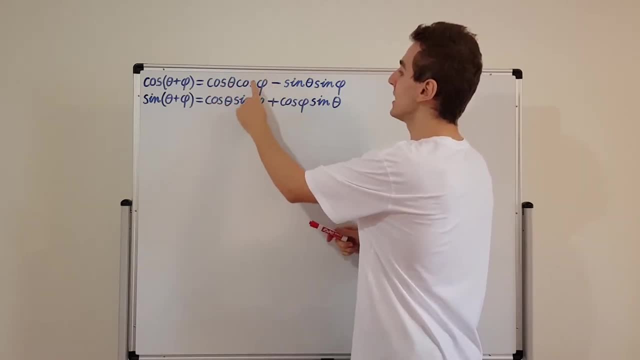 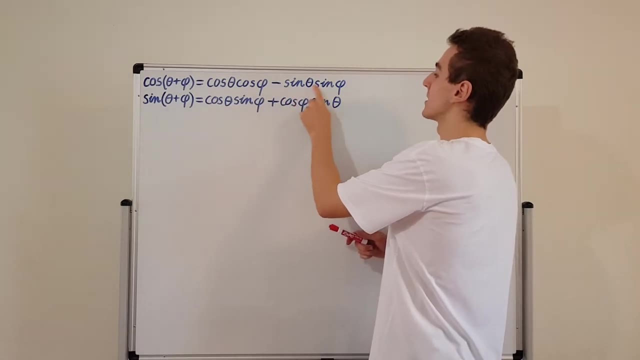 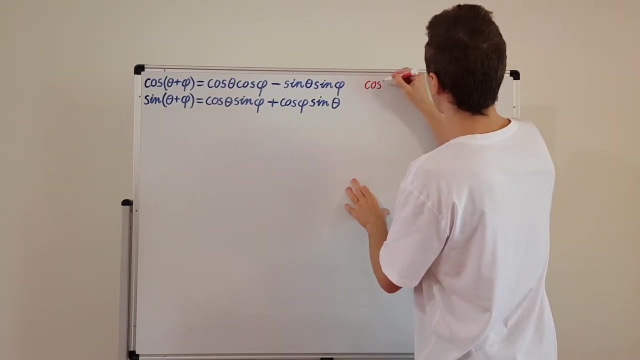 set theta equal to phi. Well, phi is going to turn to theta over here, and over here we're going to have theta. So what we're going to have is cosine theta times cosine theta sine theta times sine theta. So this is actually going to be. I'll write this out in full: we're going to have cosine of 2. 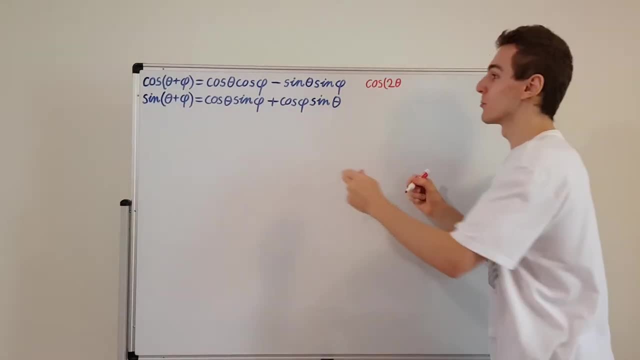 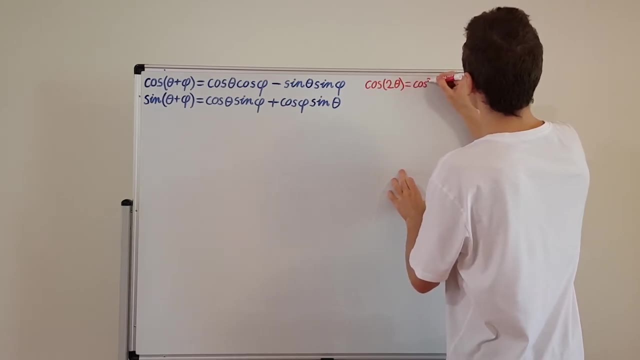 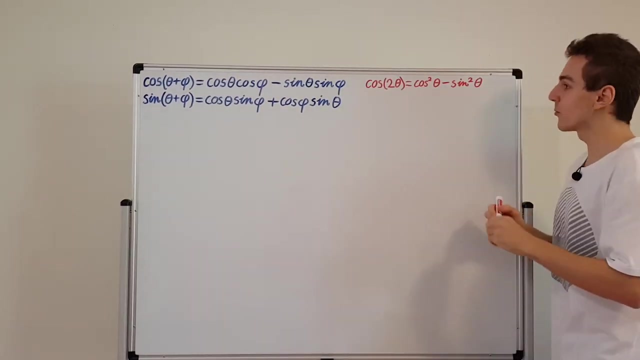 theta. right, because if we're adding the same thing, then we're going to get a factor of 2 inside. So cosine of 2, theta is equal to cosine squared of theta, minus sine squared of theta. So where does this come from? Well, it comes from this expression. So this is actually just a special case of this more. 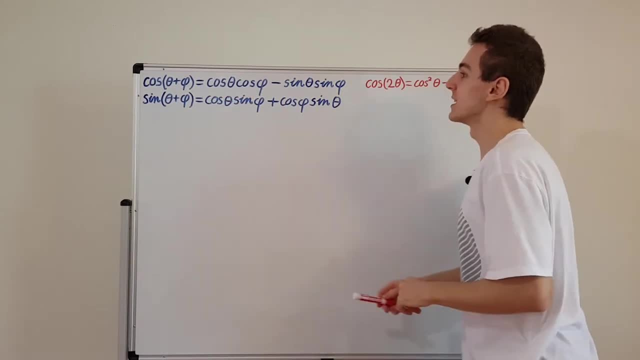 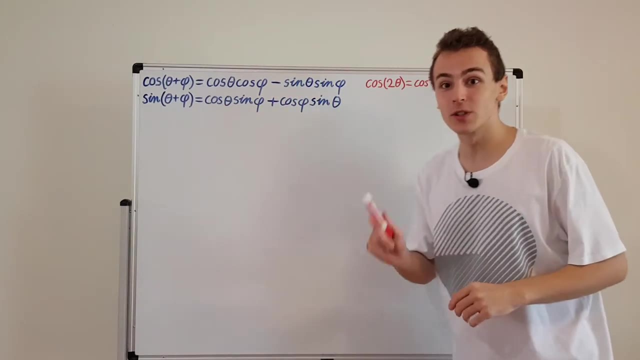 general expression. So this is a more general relationship that takes the sum of any two angles that don't necessarily have to be equal, But this guy is the special case where theta is equal to phi. So that is for cosine of 2 theta And it. 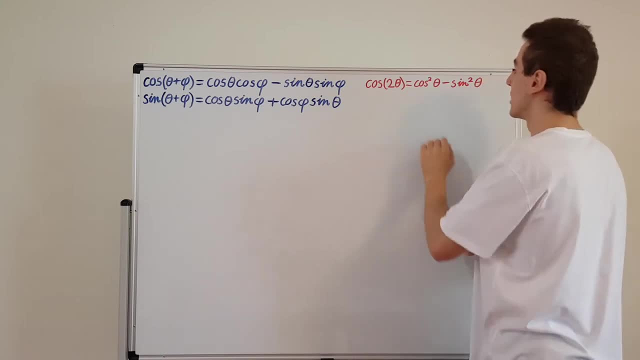 you can imagine, this is a very useful thing to deal with, because this over here can be a lot more convenient to work with than this, because here you have a factor of 2 in front of the angle, and here you're just dealing with the angle by itself. Now let's have a look at the bottom one, So the 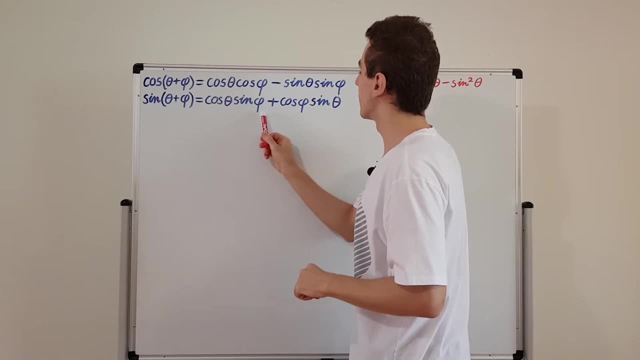 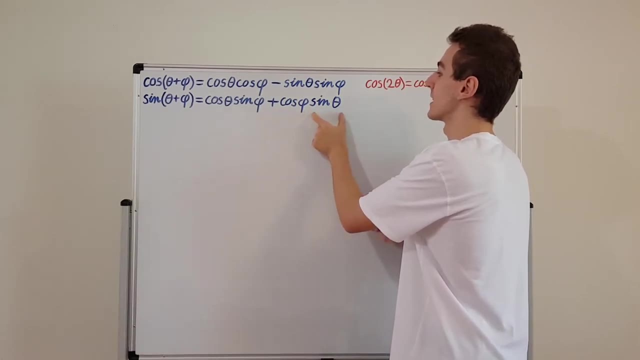 bottom one. what's going to happen to it? Well, theta and phi are going to be equal to each other, So we're going to have cos theta sine theta, and over here, we're going to have cos theta sine theta. So these guys are actually going to be the same term, So we're just going to have two copies. 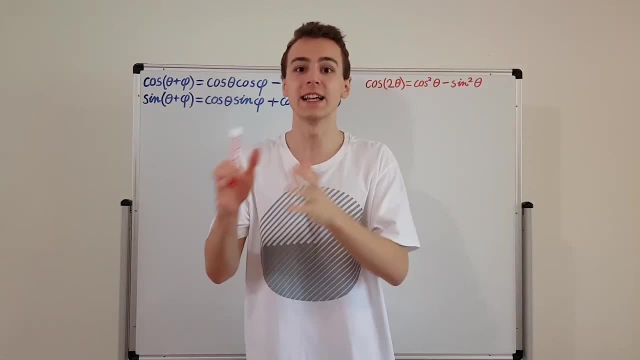 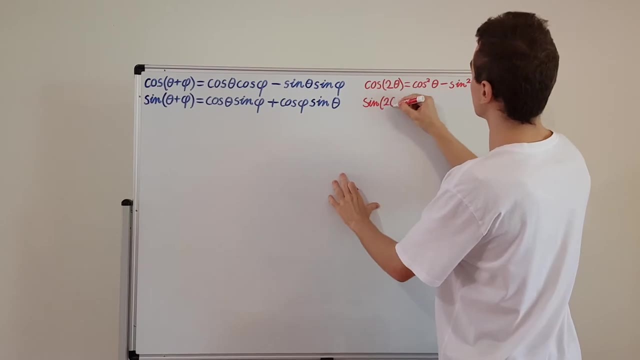 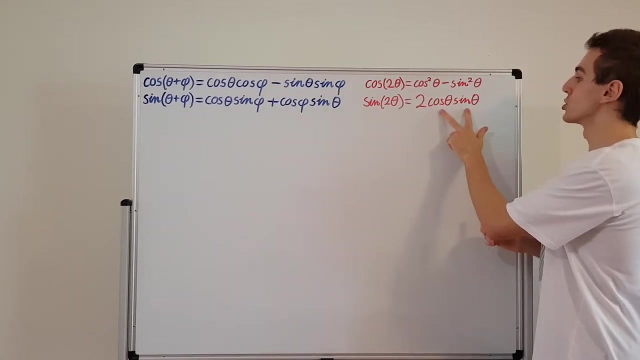 Of the same term. It's this mixed term that has cosine and sine multiplied together. So if we have sine of 2 times theta, that's going to be equal to 2 times cosine theta times sine theta. We'll have cosine theta times sine theta, And you could actually change the order of these guys around. 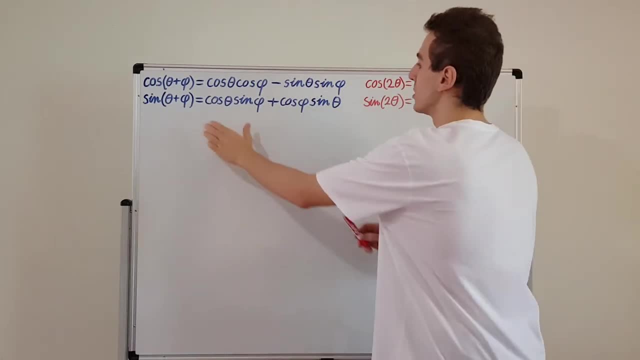 You could have sine theta, close theta. That's because multiplication is commutative, So the order over here also doesn't matter. I've just consistently put cosine to be first over here so we can keep track that theta actually gets swapped with phi in this expression. But over here. 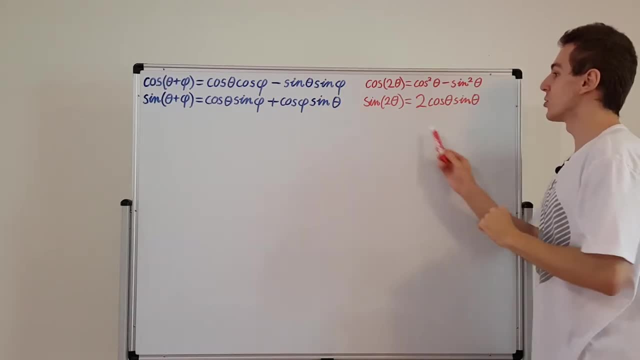 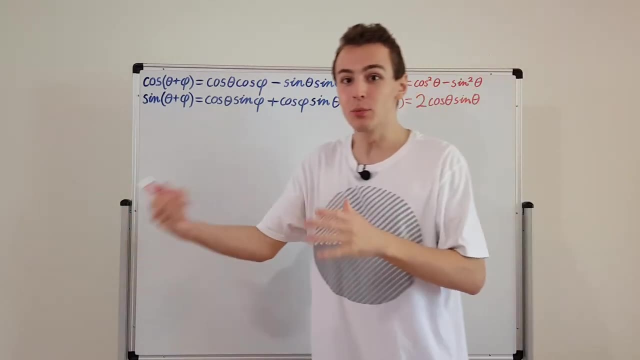 it doesn't matter, You can have cos theta or sine theta first, because there's only one angle that we're dealing with. So these guys are what happens if you take double the angle in and you input that into the cosine and sine functions. So these guys are very useful and they're just special cases. 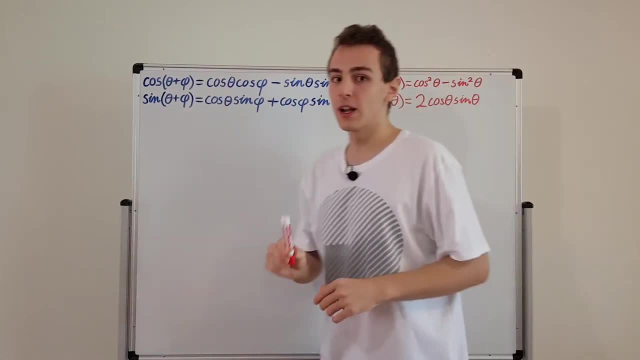 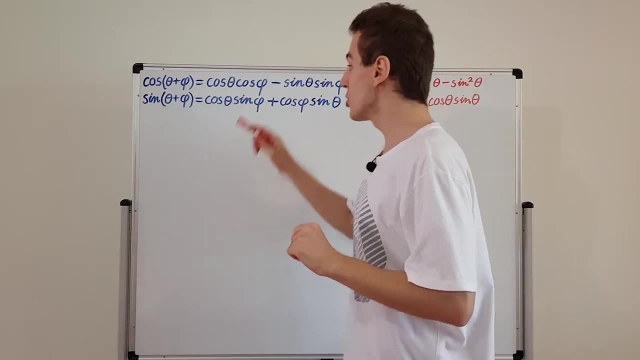 of this more general form. Now, if you remember, in the previous video which you can find in the quantum mechanics playlist- there's a link in the description below. You can also click up here. Make sure you watch that previous video, because we actually used those complex exponentials. We had something that had e to the i. 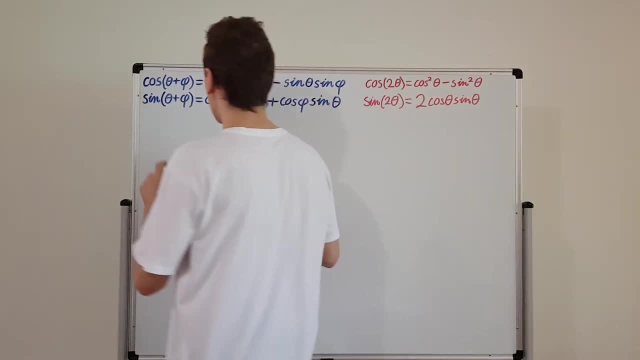 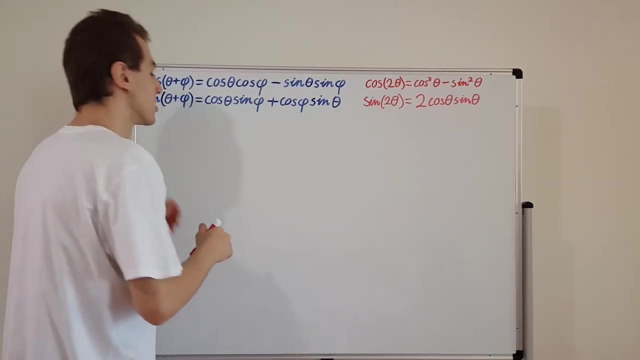 theta and e to the i phi. So what we're going to do is we're going to do a similar thing, but we're just going to do one angle. We're going to see what happens if you add an angle to itself. So if you add an angle to itself, that's the same as multiplying this exponential e to the i theta. 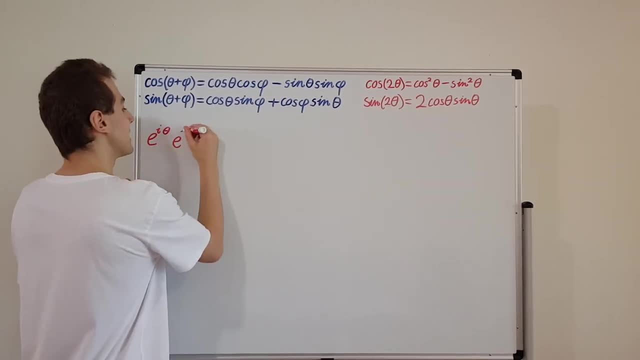 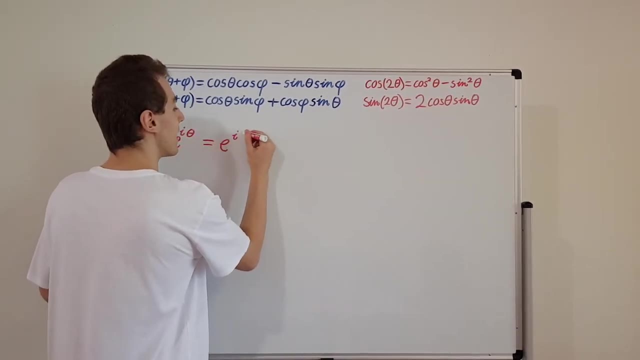 by itself. We're just going to have another copy of that. We're going to have e to the i theta. So we have this guy times this guy and that's exactly the same as e to the i theta squared. So it's like squaring this exponential and this is also the same as e to the i times 2 theta. 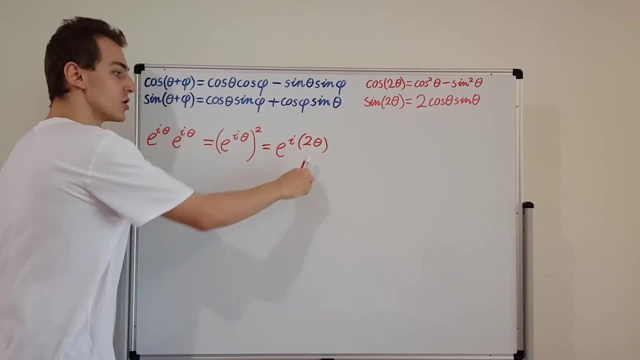 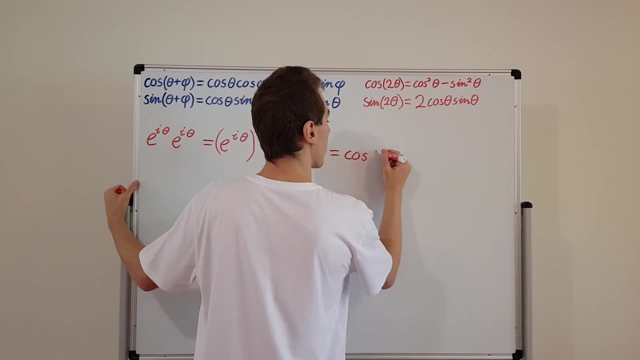 So I'll put 2 theta over here, and if you have 2 theta, we can expand this out in terms of cosines and sines, and that's going to give us cosine of 2 theta. I'm going to put brackets over here because we have more than one thing. 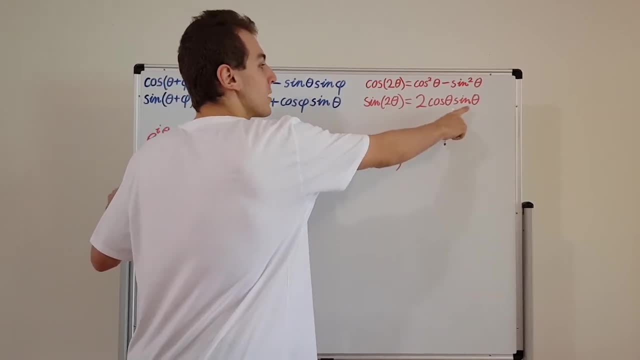 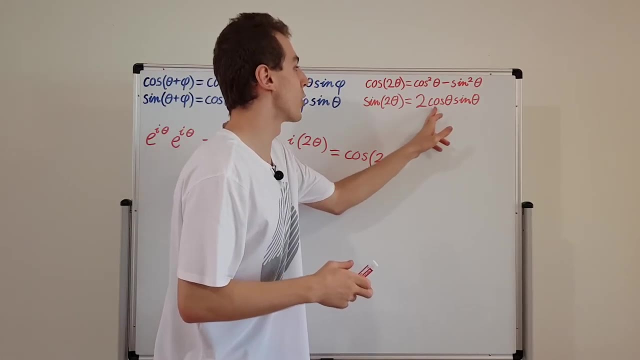 in the argument. So over here, where we have just one single angle, it's a bit redundant to put brackets because it's a bit unnecessary. You can see that theta is definitely being acted on by the cosine. There's nothing else that could be acting on the. 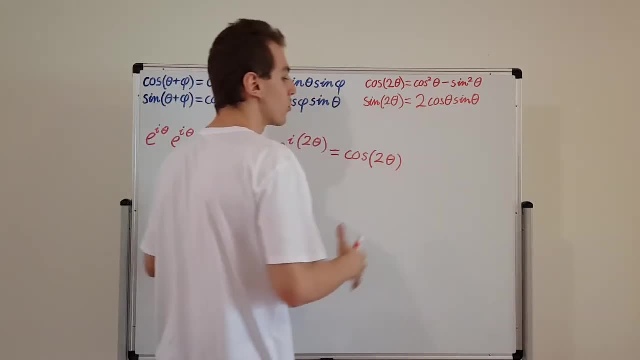 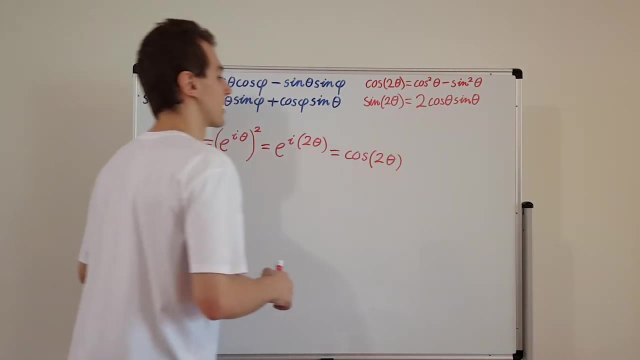 theta, But over here, because we have 2 theta, it's more appropriate to put brackets. And the more complicated your expression is, the more useful it is to have brackets. For simple expressions it's not useful to have brackets. So this is the real component, and now let's write the imaginary. 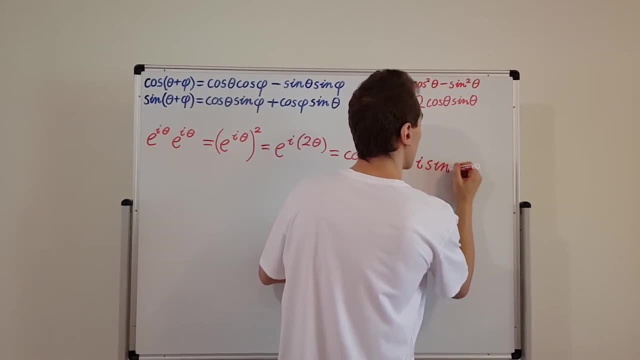 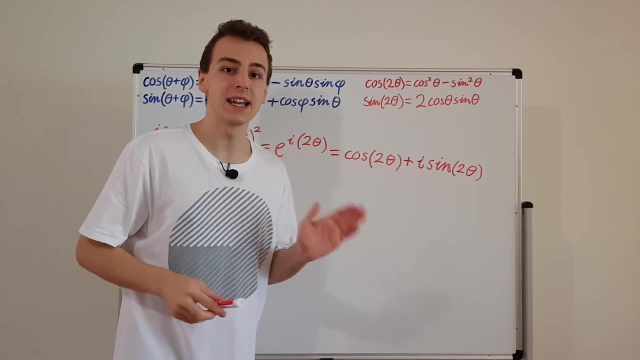 component. The imaginary component is i times sine of 2 theta. So we have 2 theta in there. So this is very similar to what we did in the previous video. In the previous video we had theta plus phi up here and then we had theta plus phi in here. 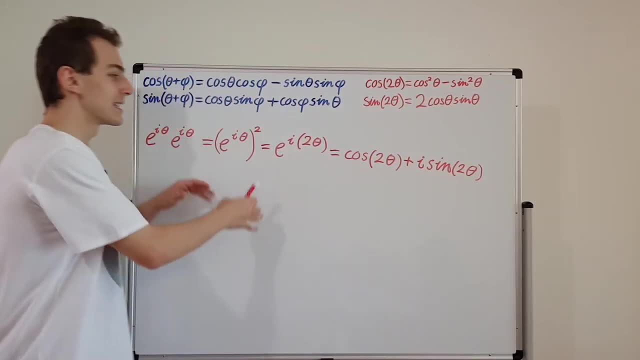 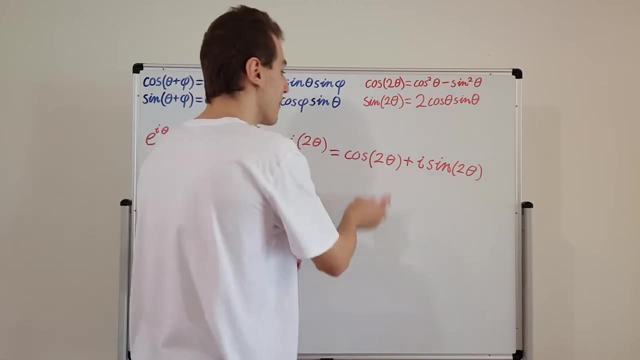 and in here. So what we're going to do now is we're going to do some algebraic manipulation and we're going to have a real component and an imaginary component and we're going to match them up again, and when we match them up, we're actually going to get these expressions. we're 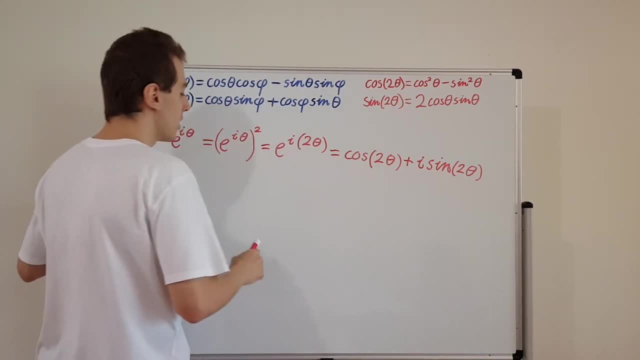 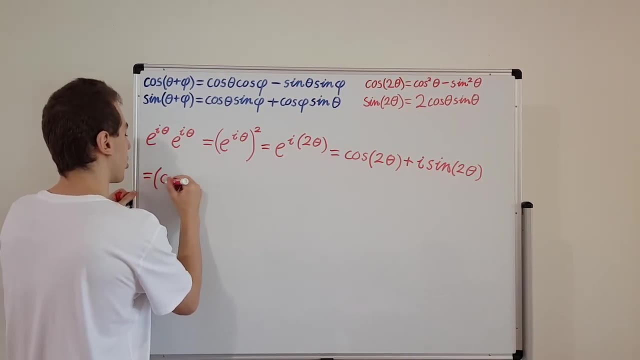 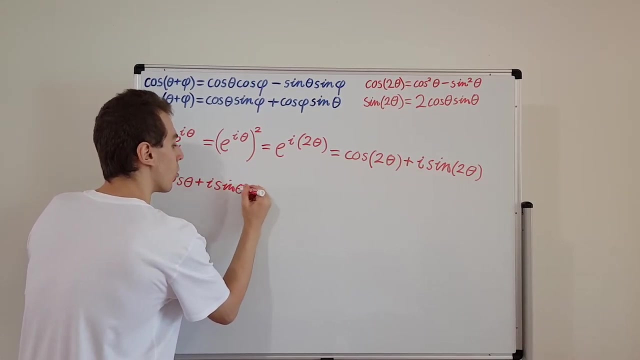 going to get the same expressions, so let's do that. we know that this guy is equivalent to just squaring. it's the same as going cos of theta, because that's that's what this exponential is. the same as cos theta. i sine theta, all squared right. that's, that's exactly what this thing is. 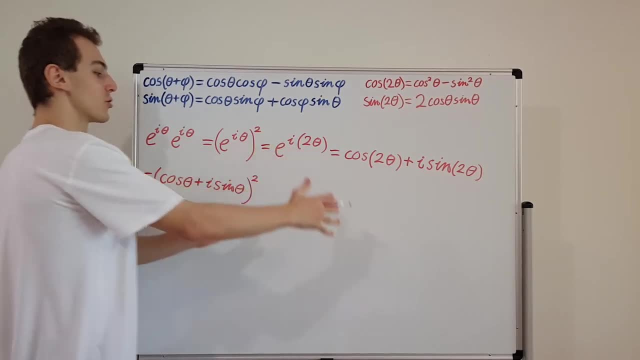 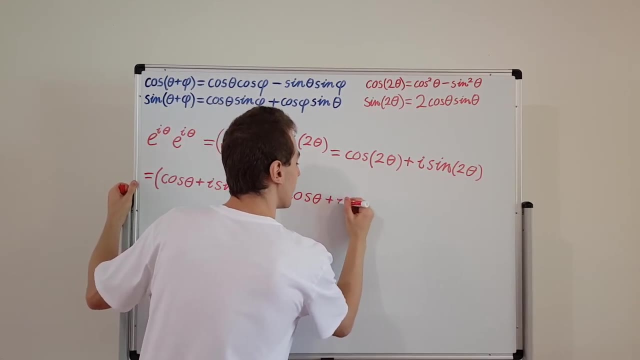 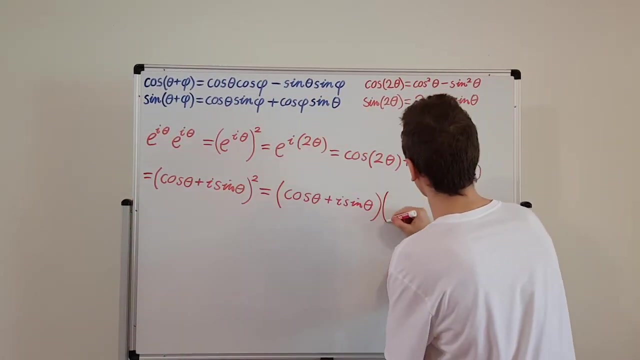 and we know this is actually the same as just multiplying that exponential by itself. so i'll write that out in full. so we have cosine of theta plus i sine theta. we're going to have another copy of that. i'll write it over here. this is just so we can keep track of which terms are where. 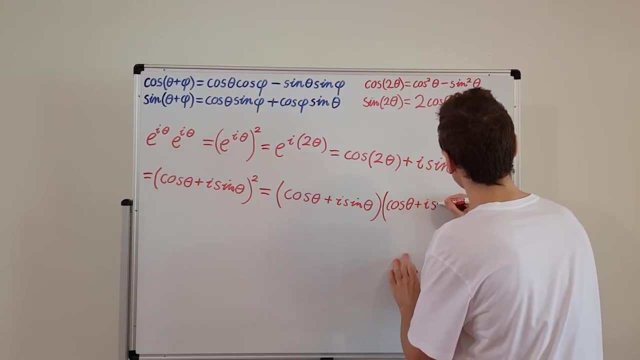 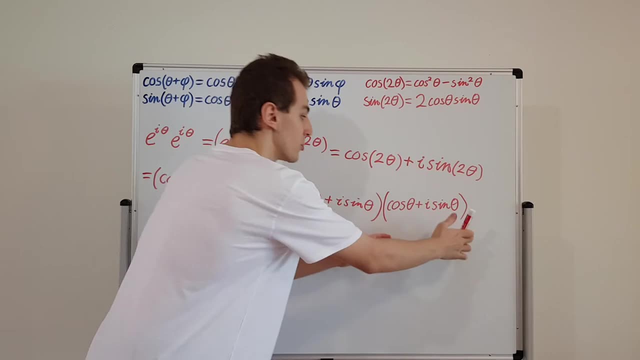 so we have cosine of theta plus i sine of theta, so we have two copies of that. right, we're squaring and i've written it out in full so we can match up all the terms. i'm going to write that below and we're going to get an expression that has a real 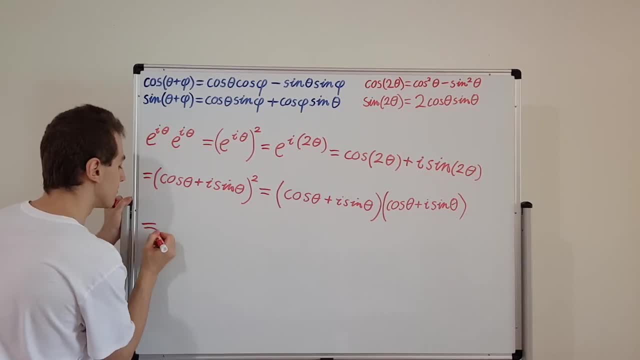 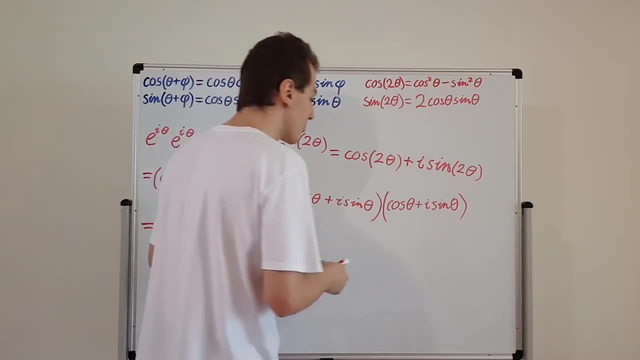 component and an imaginary component. so that is equal to what's our real component going to be. so a real component is going to have no i's in it and the imaginary component is going to have a single i multiplying every, every term in there. so how are we going to eliminate the i's? well, 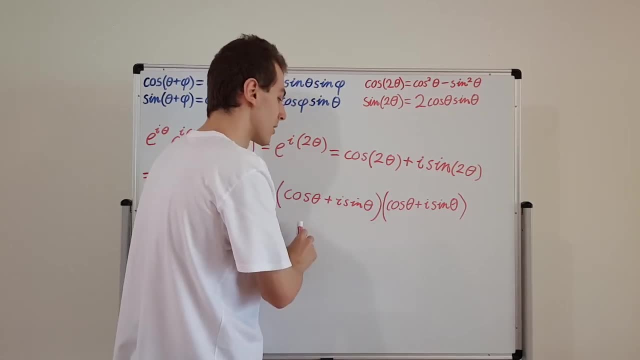 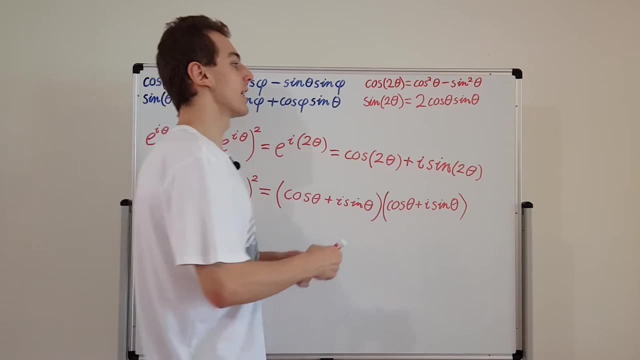 this term and this term they don't have any i's, so that's going to be real. this term multiplied by this term, that's going to have an i times an i, which is i squared, and i squared is minus one, so i squared is equal to minus one, so we can get rid of that. 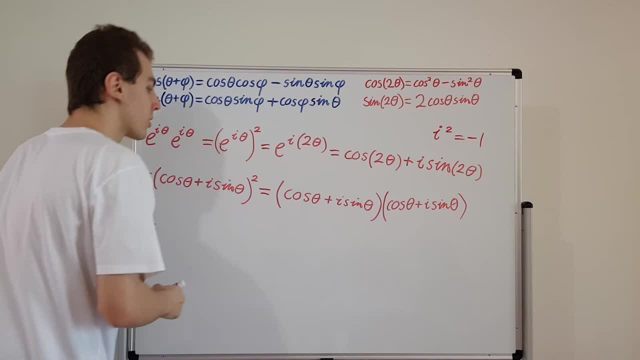 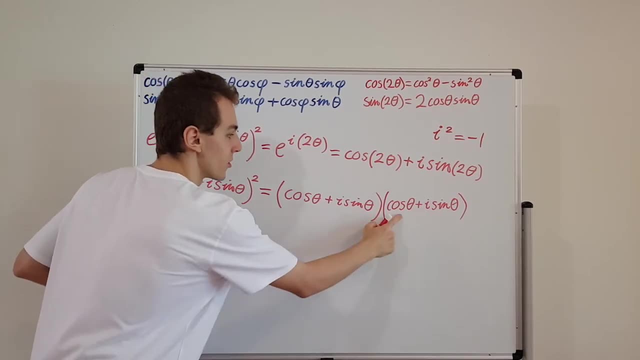 i. by multiplying it by another: i. so what's our real component gonna be? well, the real component is gonna be cosine squared of theta. that's what we get from the first terms being multiplied and the last terms being multiplied together. it's i sine theta times i sine theta. 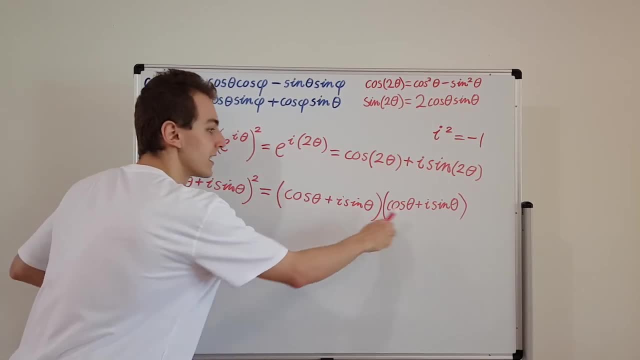 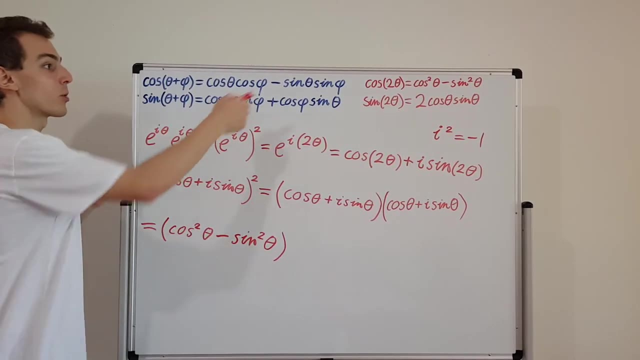 the i squared is going to become minus one, and the sine times sine is going to be sine squared theta. Now this should look familiar. This is what we have up in the top right corner. This guy is exactly the same as this guy. So now let's have a look at the. 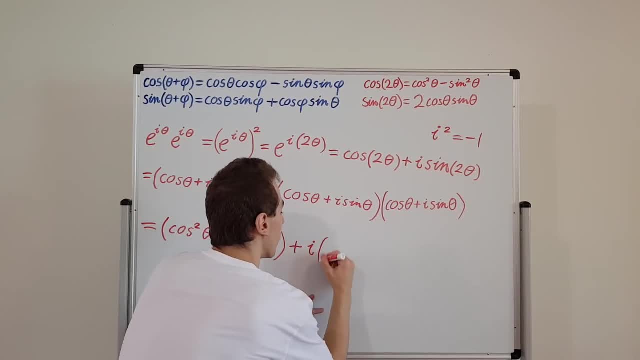 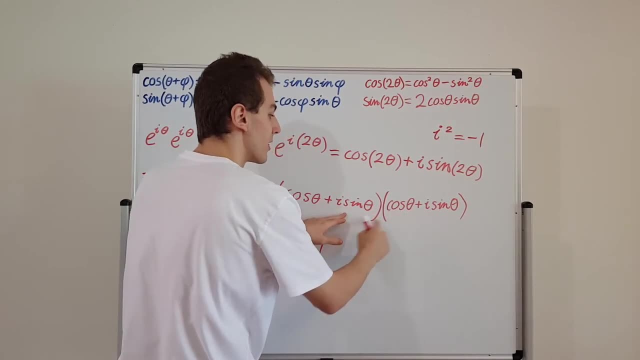 imaginary component. The imaginary component is i multiplied by what is the imaginary component? Well, it's going to be the mixed terms. We're going to have sine theta, cos theta from this term over here, and we're also going to have cos theta times sine theta. So these are actually the exact same. 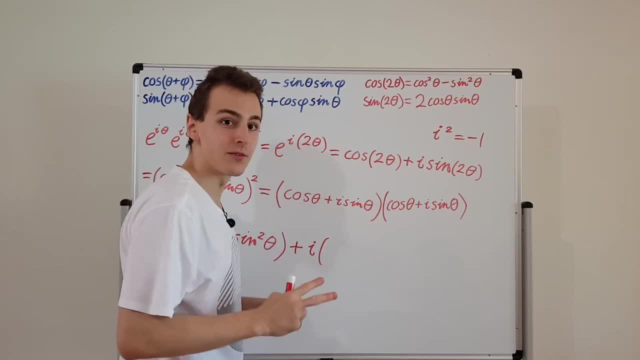 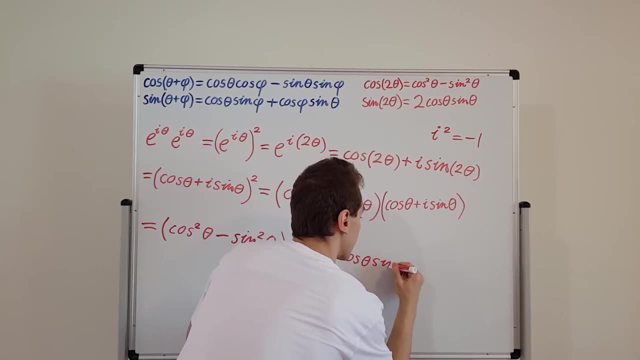 term. This and this are exactly the same. So we're going to have two copies of them. and if we have two copies, we're going to write a factor of two and then we'll have cosine theta and sine theta. So those are the two copies from these mixed terms. That's these outer terms and these inner terms. 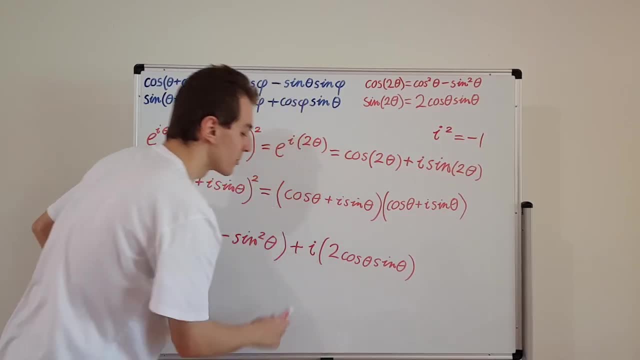 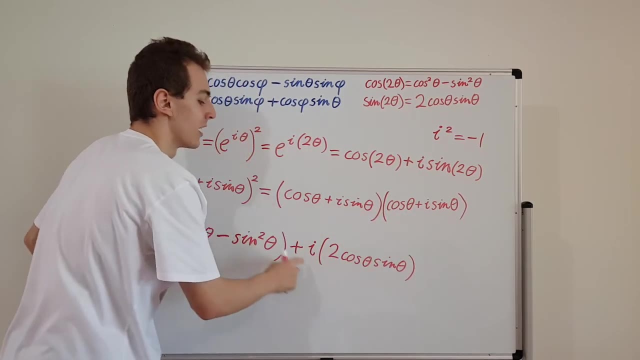 And this is the imaginary component, It's the term that gets multiplied by i, because both of these guys introduce one copy of i. We have one i over here and we have one i over here and we can factor that out and that's going to give us this. 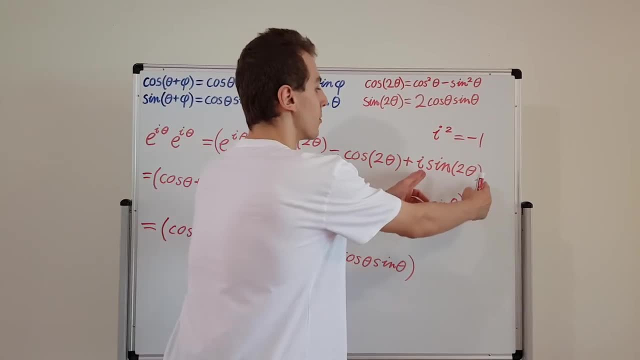 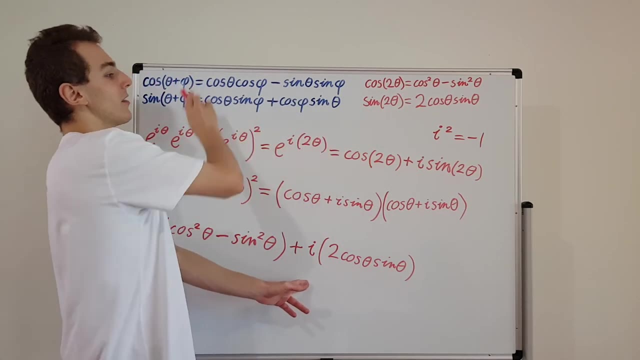 So this you can identify with the imaginary component, Sine of 2 theta is 2 cos theta sine theta, and that's what we have over here. That's the special case of this thing that we derived in the previous video And the real component. you can identify, this expression cos squared. 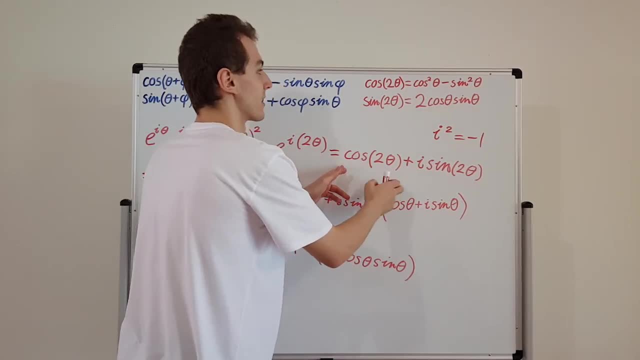 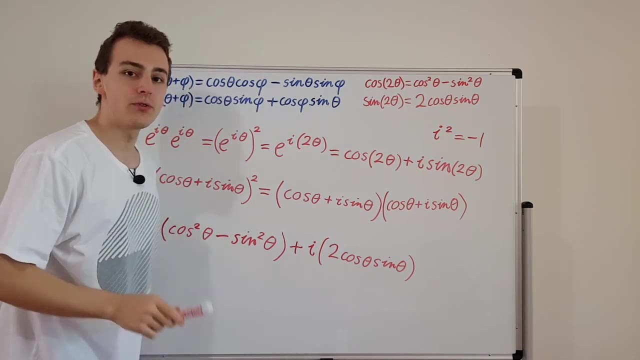 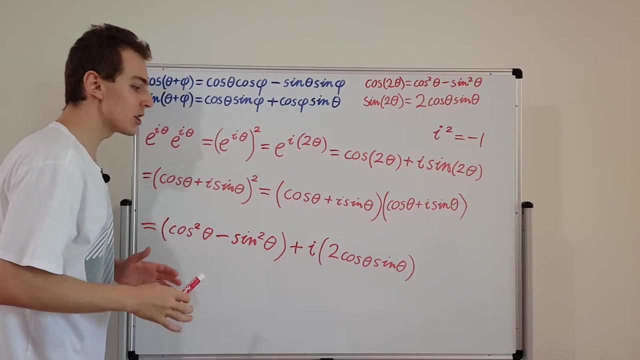 theta minus sine squared theta, That is the same as cos of 2 theta and that's what we have written up here. So we've derived these two trigonometric identities using two different techniques. We've done it using complex numbers, So we started with e to the i theta and we've done some algebraic manipulation and we've actually 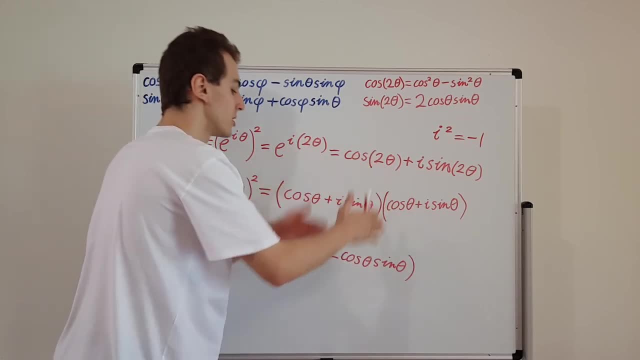 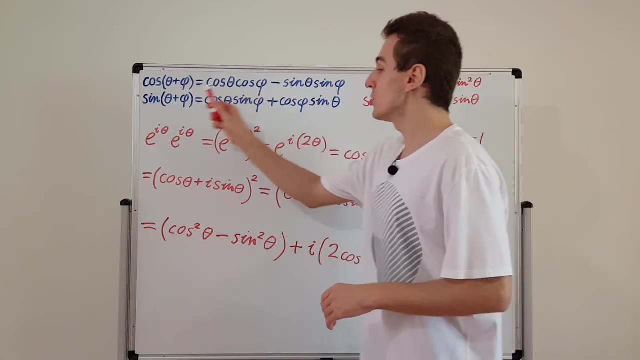 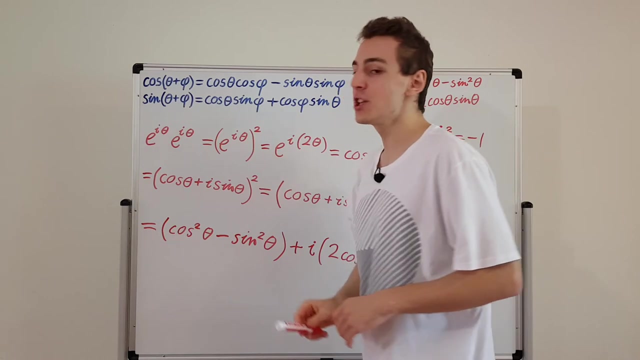 assigned these real components to each other and these imaginary components to each other. That's the same logic as the previous video, And the alternative derivation that we actually used at the beginning of the video was using these other trigonometric identities, which are more general, and then we've simplified them by imposing the condition that the angles have to be equal to.